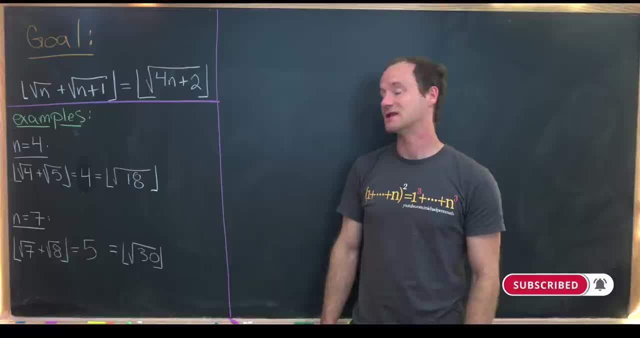 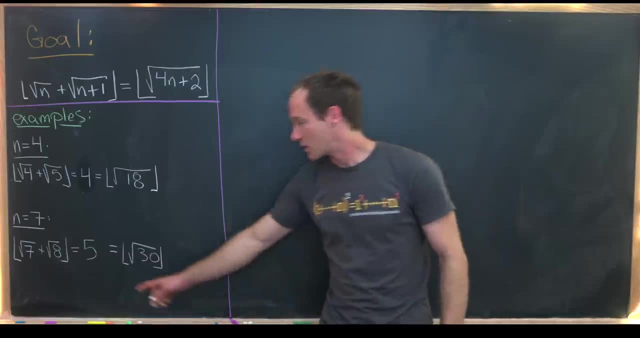 because the square root of 18 is bigger than 4, but it is less than 5.. Now, similarly, we can look at n equals 7.. So over here we have the square root of 7 plus the square root of 8.. 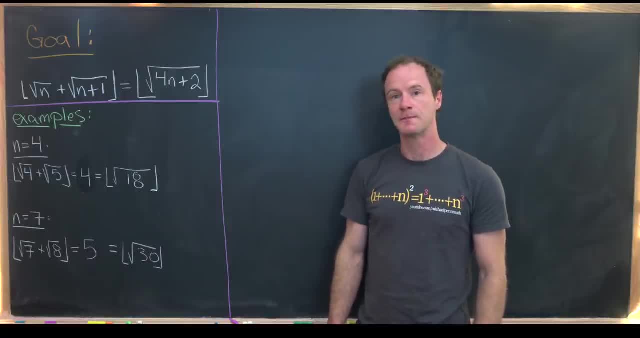 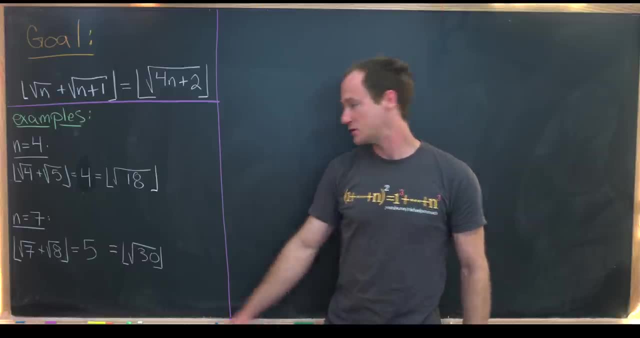 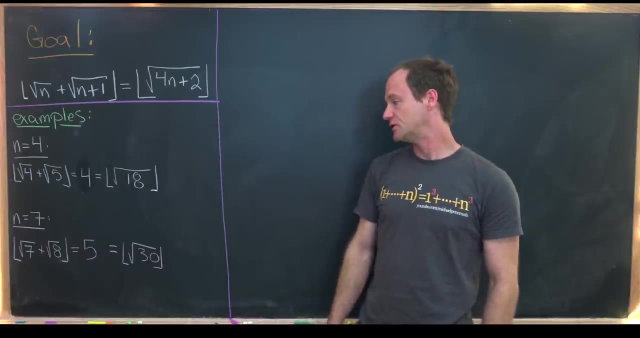 So those are both between 2 and 3,, but they add up to something which is bigger than 5, but less than 3.. So that means, when you take their floor, you get 5.. Furthermore, if you plug n equals 7 to this 4n plus 2,, you get 30. 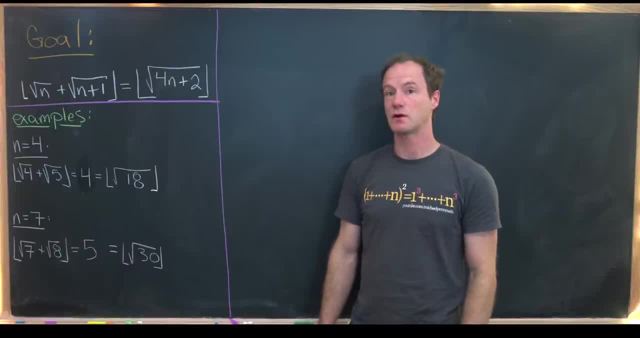 Well, the square root of 30 is going to be bigger than the square root of 25, but less than the square root of 36.. So it'll be between 5 and 6.. You take the floor and you'll get 5.. 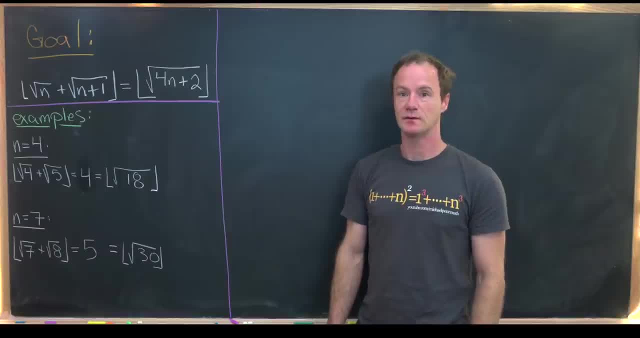 So you have the same thing on either side there too as well. Okay, so now that we've looked at some examples, let's go ahead and see if we can solve this, Or I should say, we can show that this equation is true. 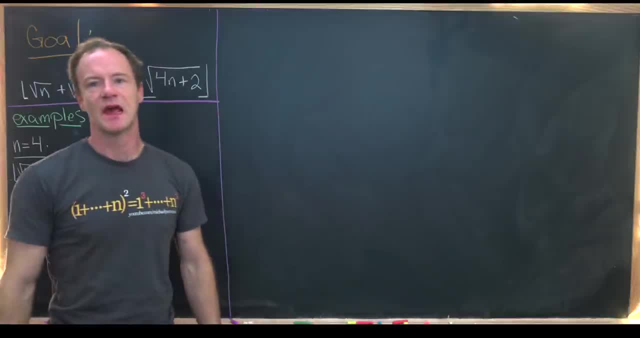 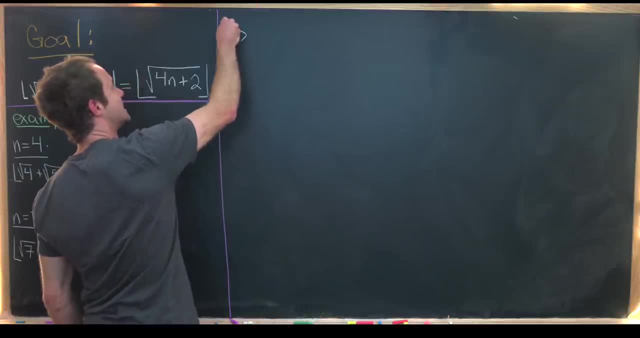 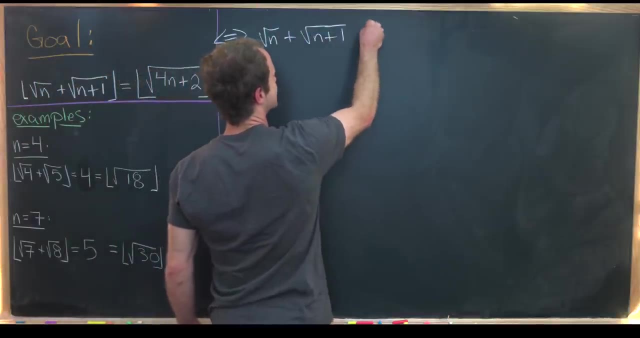 So we'll start by taking our equation and rewriting it as something that is equivalent, using some tricks about perfect squares. So this equation is equivalent to saying that the square root of n plus the square root of n plus 1 is on some suitable open interval. 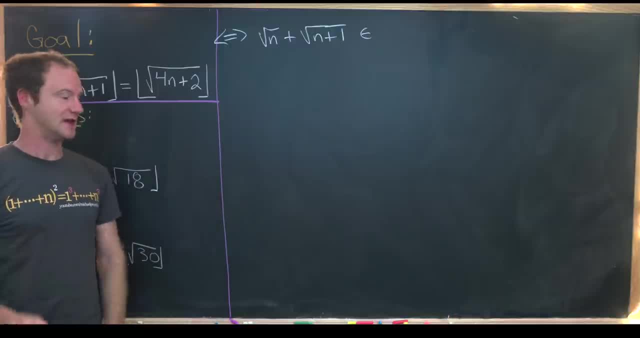 So we can say that it's on an open interval bound by integer, because it's impossible for n and n plus 1 to both be perfect squares, So it has to be on the interval from the square root of 4n plus 1. 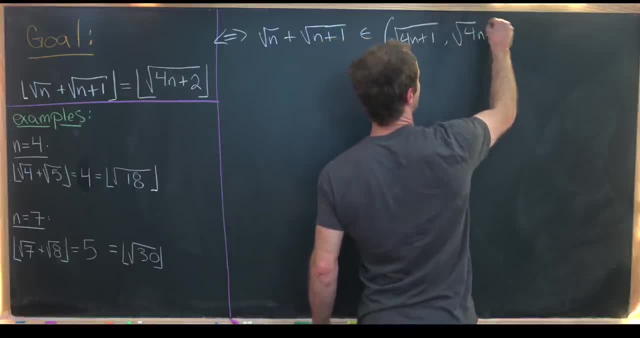 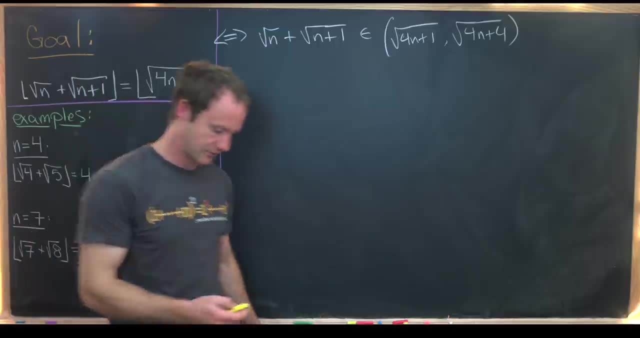 all the way up to the square root of 4n plus 4.. And you might say: well, what about the square root of 4n plus 2 or the square root of 4n plus 3?? Well, it's well known that 4n plus 2 and 4n plus 3 cannot be perfect squares. 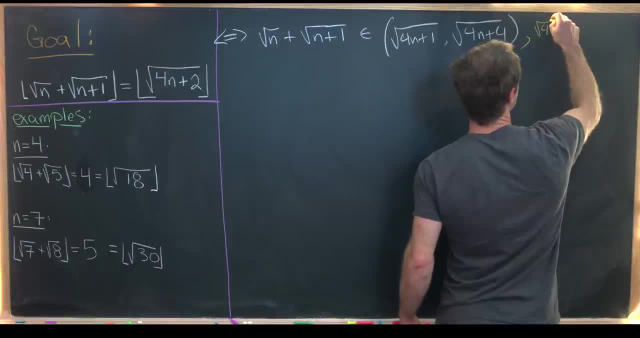 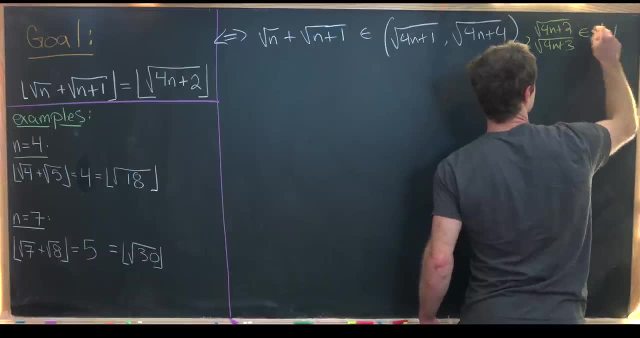 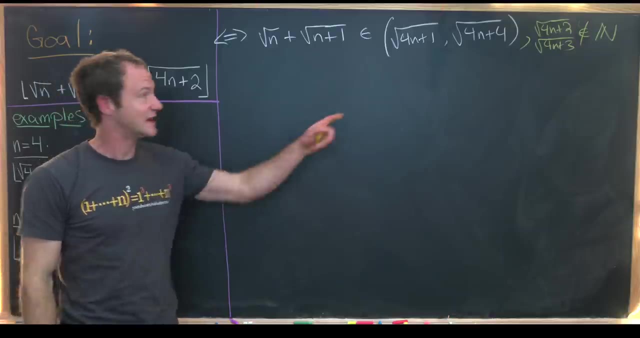 So that means that the square root of 4n plus 2 and the square root of 4n plus 3 cannot be whole numbers. So I'll just write: they cannot be natural numbers. So since those can't be natural numbers, we don't need to consider them as endpoints inside of our interval there. 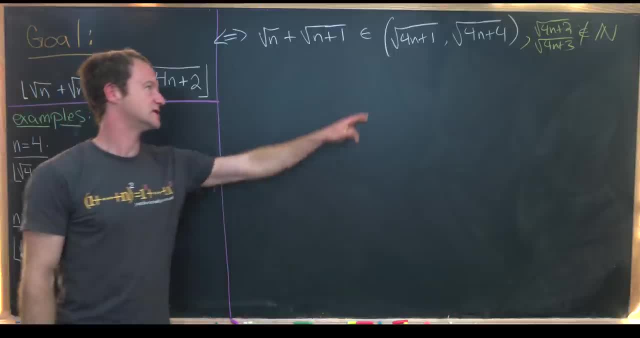 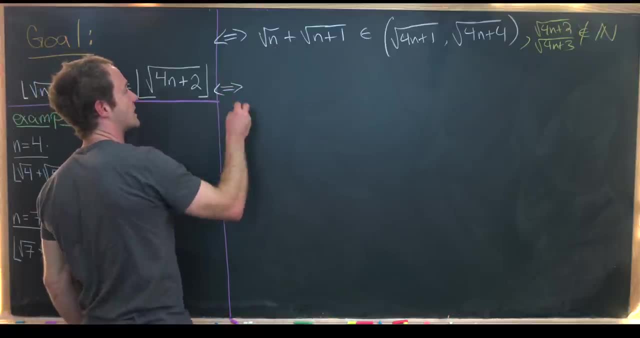 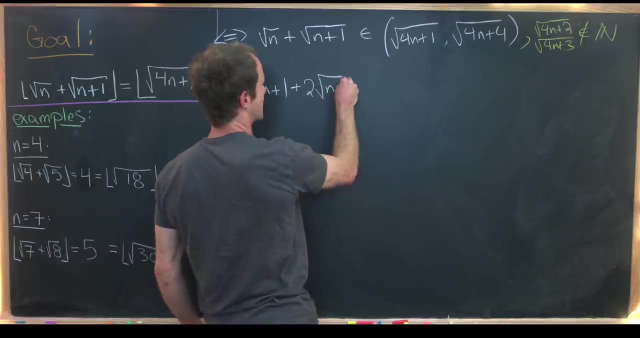 Okay. so now let's maybe square this so that we're dealing with an interval over here, with endpoints which are whole numbers. So squaring this will give us 2n plus 1 plus 2 times the square root of n times n plus 1.. 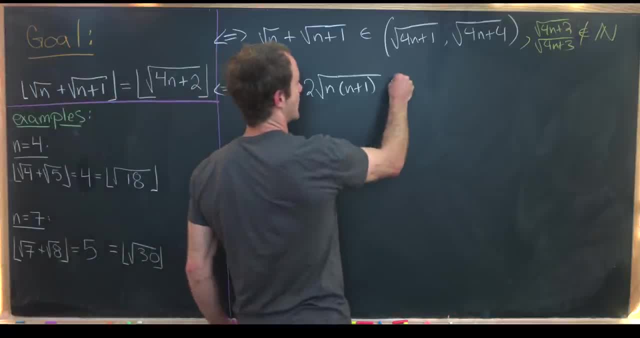 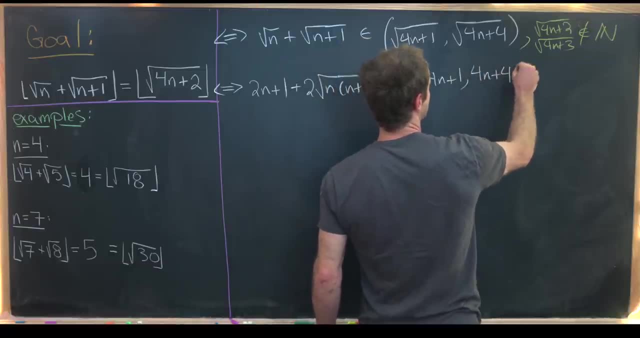 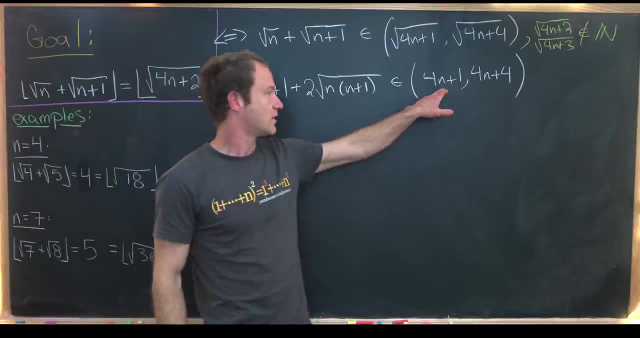 That's just squaring that like a binomial And then squaring each of these endpoints. we'll have 4n plus 1 here and then 4n plus 4 here. Okay, great. Next, what we'll do is subtract 4n plus 1. 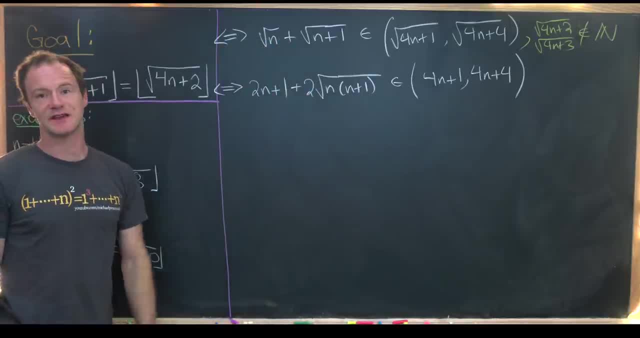 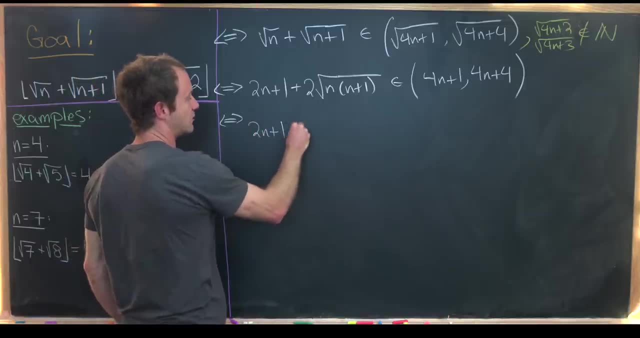 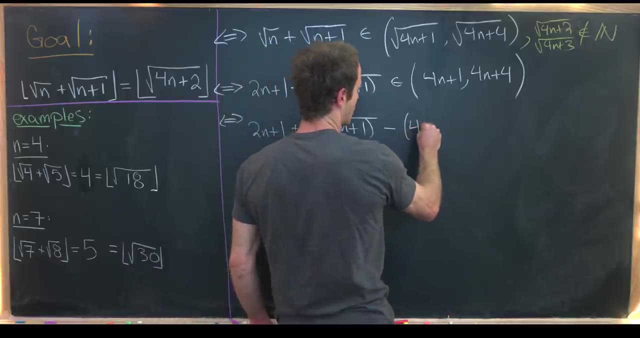 4n plus 1.. from either of these endpoints and this left-hand side of the inclusion. So this is going to give us 2n plus 1 plus 2 times the square root of n times n plus 1 minus 4n plus 1. 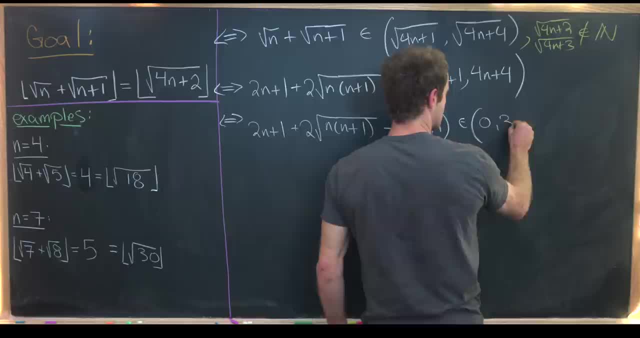 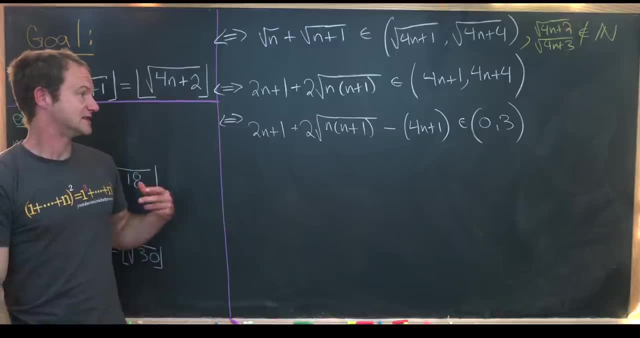 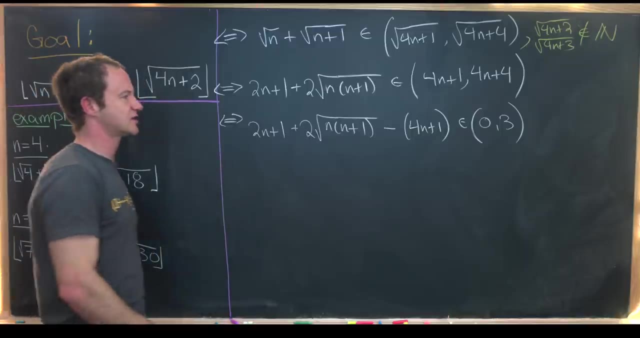 is an element of the interval from 0 to 3.. So just to reiterate, what we've shown is that our equation is equivalent to showing this object is on the interval from 0 to 3.. So now let's start simplifying this object. 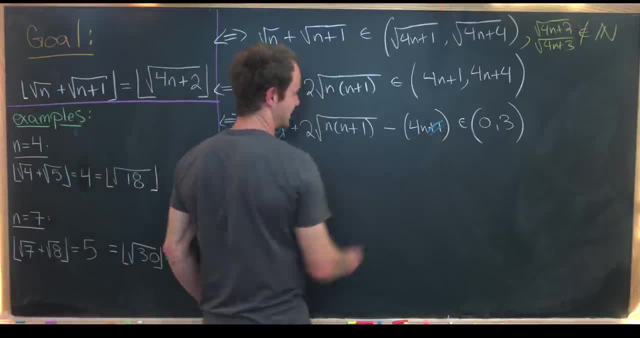 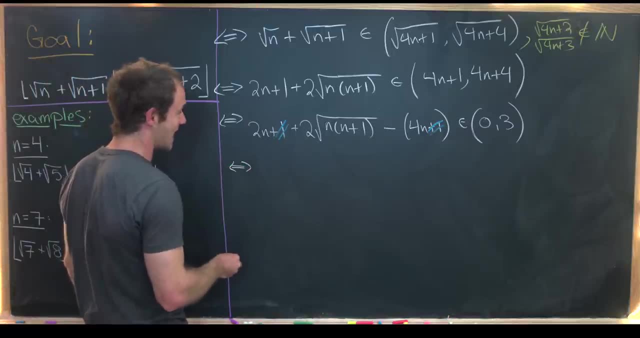 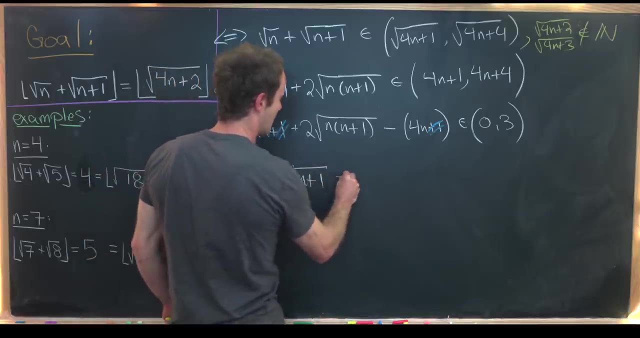 Notice that this 1 and this 1 can cancel because they have opposite signs, And then we have 2n minus 4n. So this is equivalent to saying that 2 times the square root of n times n plus 1 minus 2n, is on the interval from 0.. 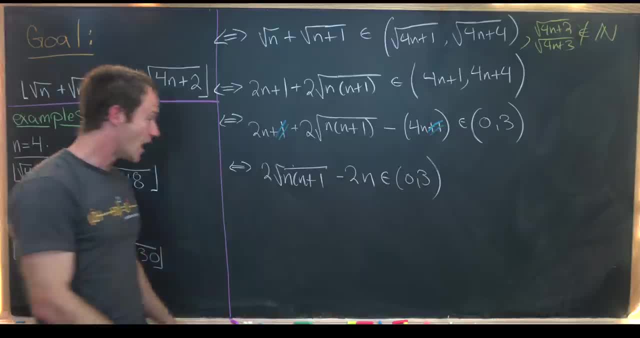 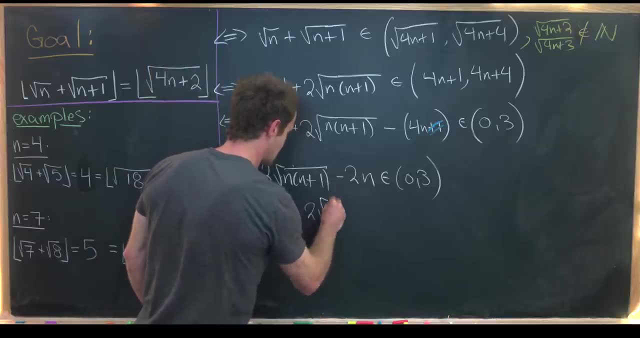 So this is equivalent to saying that 2 times the square root of n times n plus 1 minus 2n is on the interval from 0 to 3.. In other words, this is the same thing as showing that 0 is less than 2 times the square root of n. 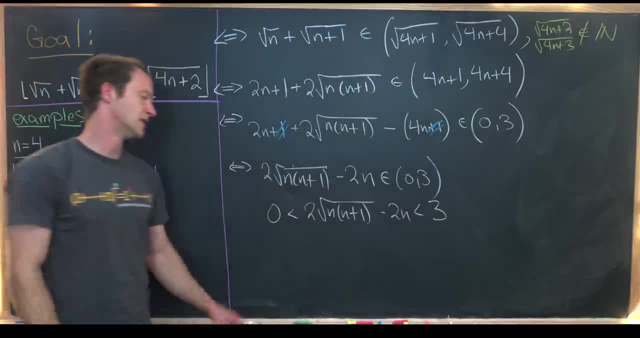 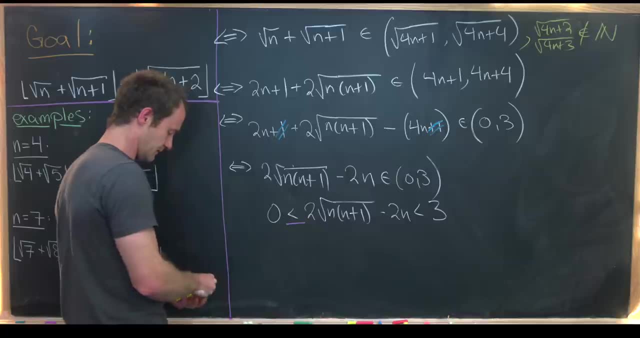 times n plus 1 minus 2n, which is less than 3.. So now we just have to tackle each of these inequalities. We need to show that this inequality is true and this inequality is true. Okay, So let's see if we can do that. 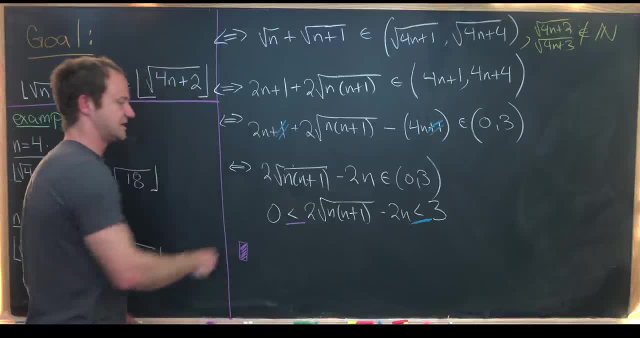 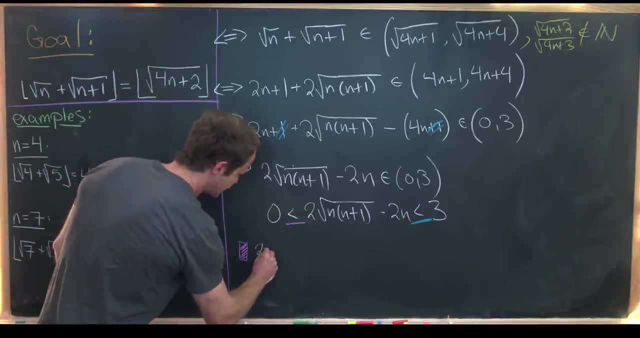 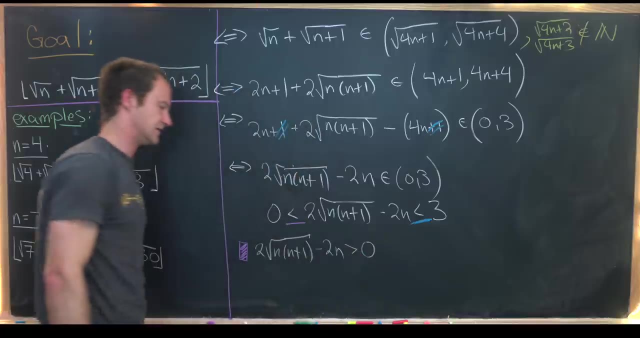 Maybe here I'll put a purple square to say that we're showing that that inequality is true. Okay, So let's notice that 2 times the square root of n, times n plus 1 minus 2n being bigger than 0, I just moved things around a little bit. 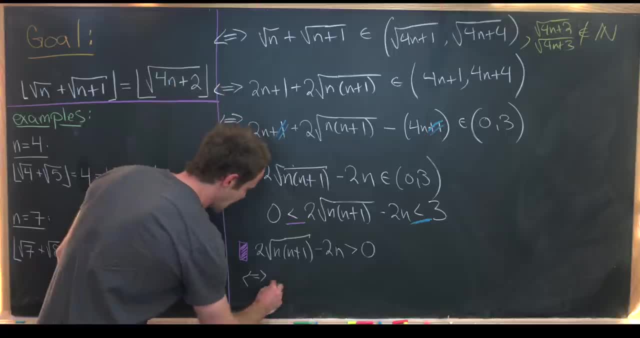 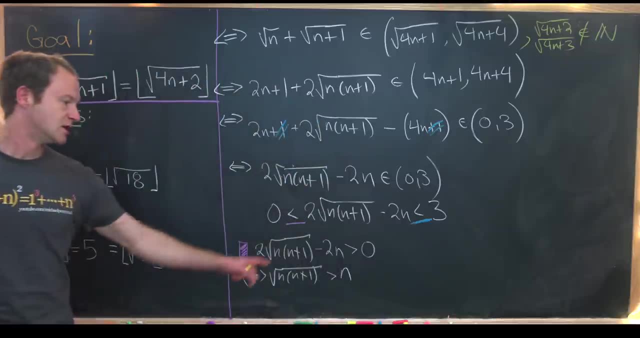 is equivalent to saying that the square root of n times n plus 1 is bigger than n. So I've moved my 2n over to the other side of the equation and then I've divided by 2.. But now we can square both sides. 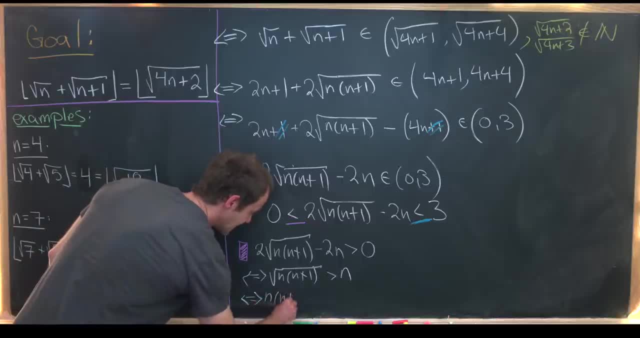 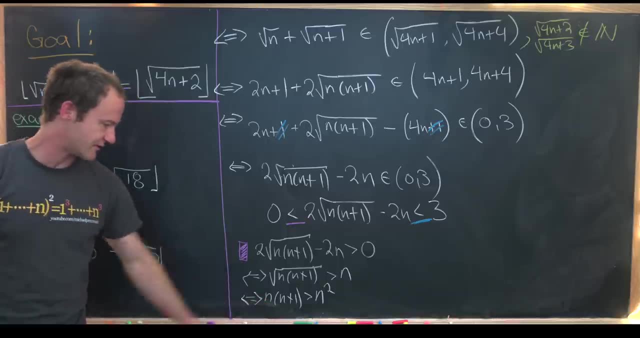 and say that this is equivalent to n times n plus 1 is bigger than n squared. But that's clearly true, because over here we have n squared plus n. n squared plus n is clearly bigger than n squared, especially when n is bigger than n squared. 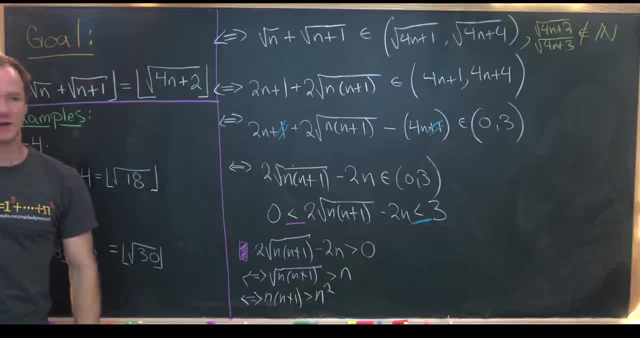 n is a natural number which we're kind of assuming over here without explicitly saying it. Okay, So that means we have achieved this inequality here. Now we're ready to move on to the second inequality, which I have color coded here in blue. 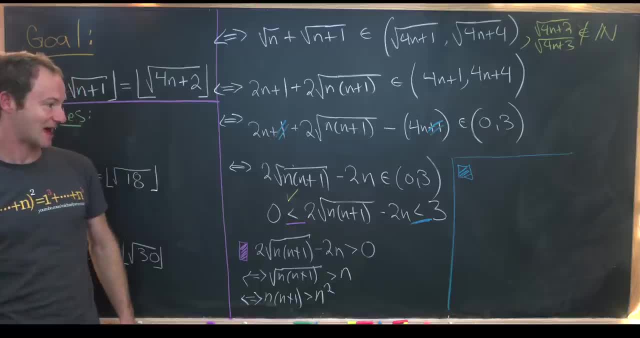 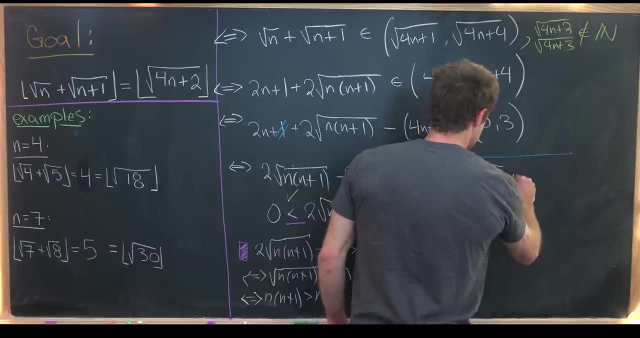 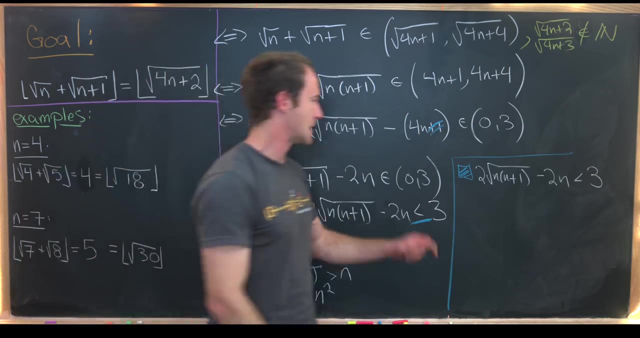 So I'll make my blue box here to say that I'm testing that inequality. So in other words, I want to show that 2 times the square root of n, times n plus 1 minus 2n is less than 3.. Okay, 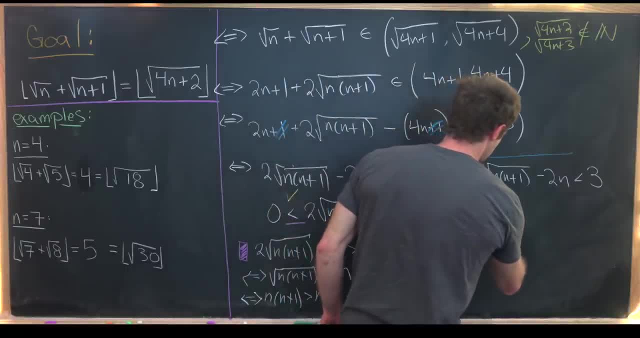 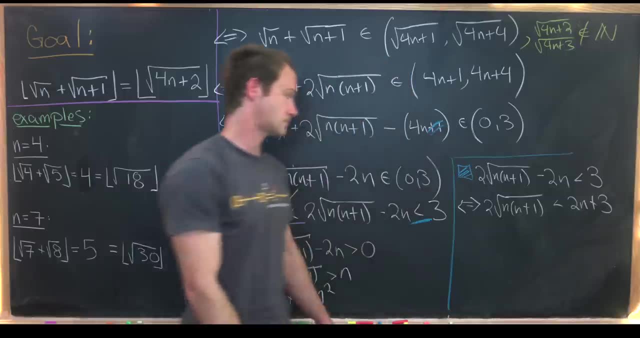 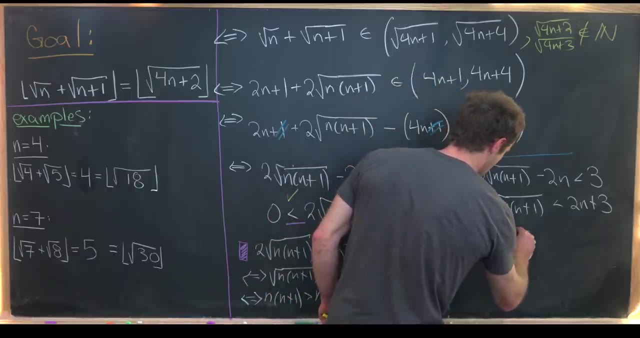 Well, that's going to be equivalent to saying that 2 times the square root of n times n plus 1 is less than 2n plus 3.. And now I can square both sides, So that'll be equivalent to 4 times n squared plus 4n. 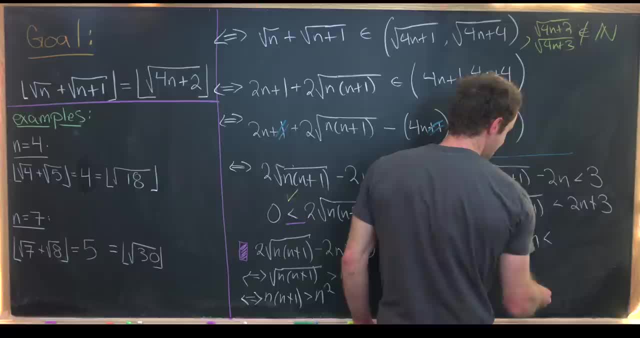 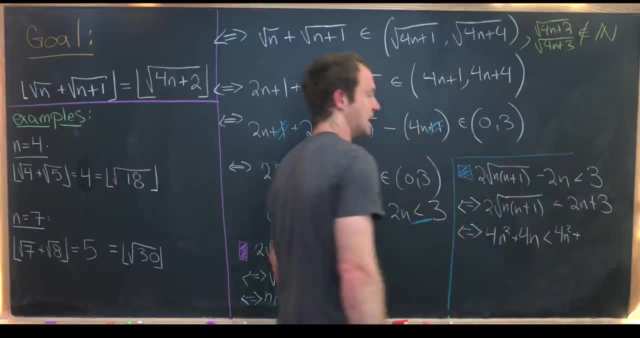 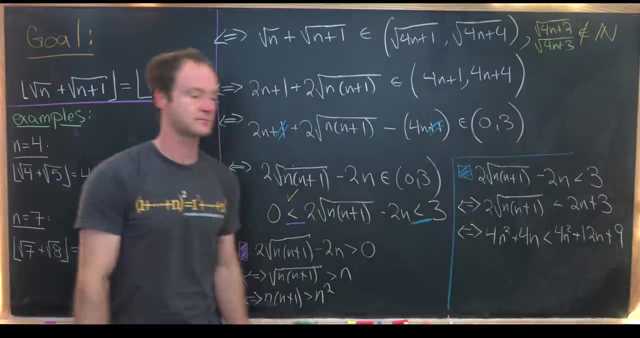 That's what we get, for the left-hand side is less than 4n squared plus. Well, let's see what we get here. We get 2n times 3 plus 2. So that'll be 12n plus 9.. 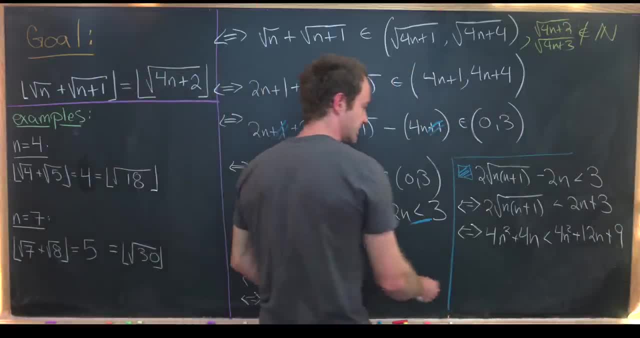 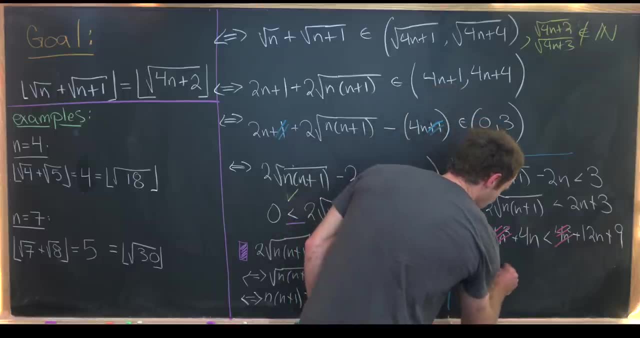 But now we can do some cancellation here. So notice that this 4n squared will cancel this 4n squared. Then we can move that 4n over and we get that. this is equivalent to saying that 0 is less than 8n squared. 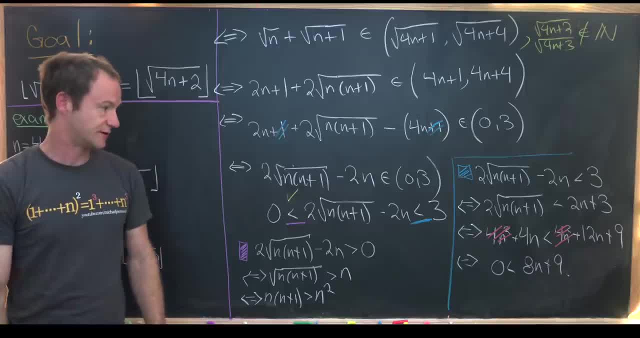 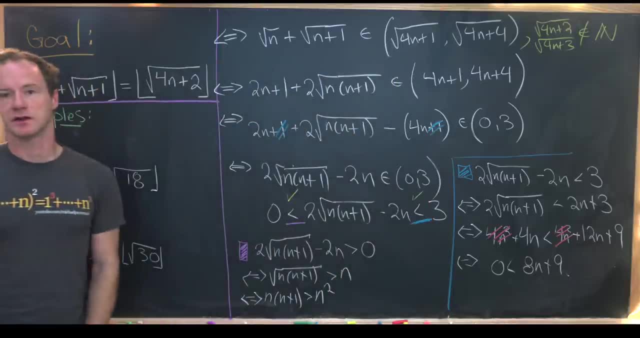 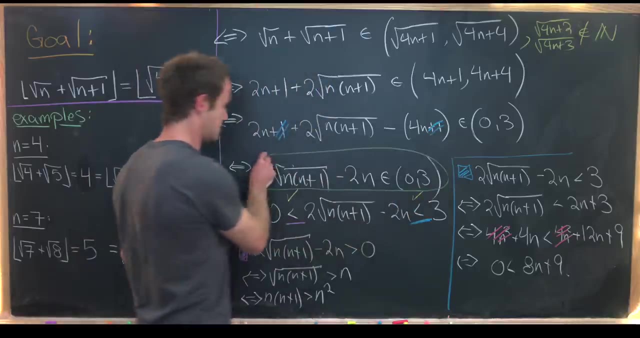 Plus 9.. But again, that's obviously true for natural numbers, so we're good to go there as well. So we've established this portion of the inequality, But that means that we've established this inclusion inside of the interval from 0 to 3,.